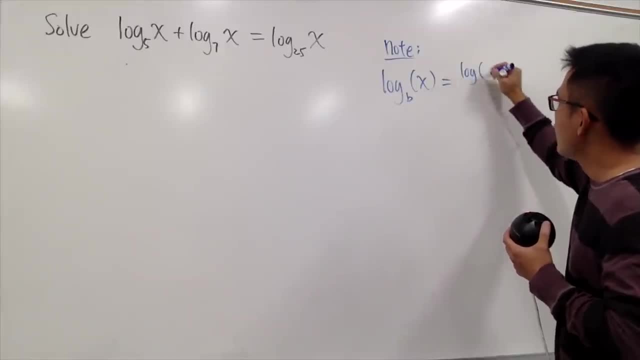 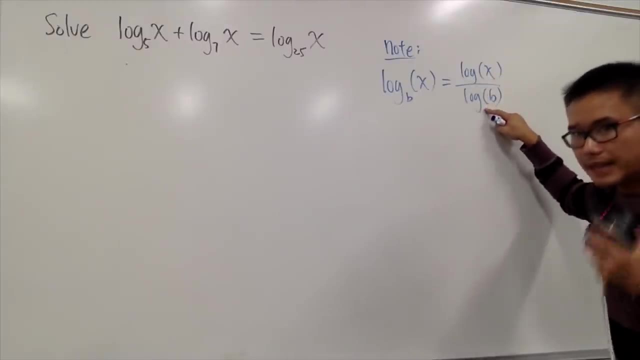 This right here. we can write this as log of x over log of b. And you see, I didn't put down any numbers here, because I'm just taking log base 10, log base 10.. As long as these two are the same, it's okay. 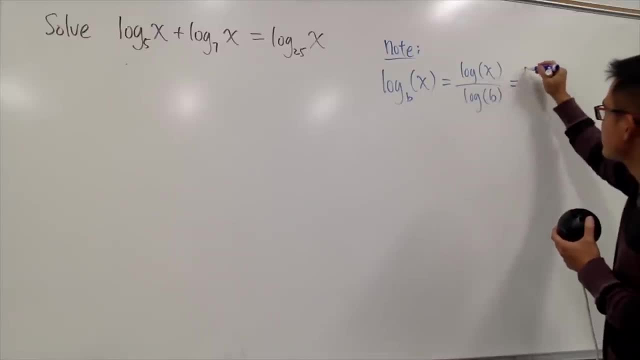 If you would like, you can also take the natural log right, So you can also do this as the natural log of x over the natural log of b right. You can also do it with log base 3 of x Over log base 3 of b. 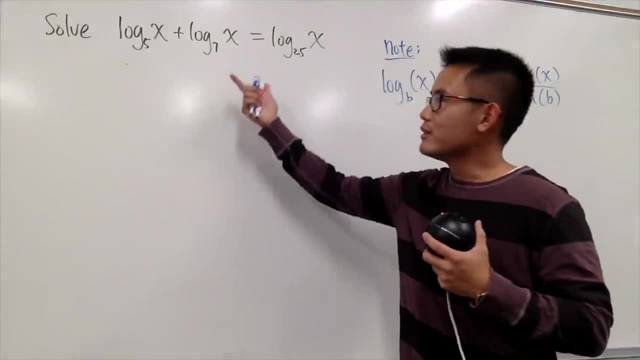 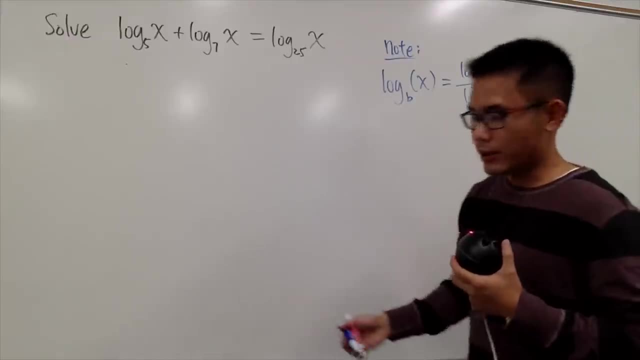 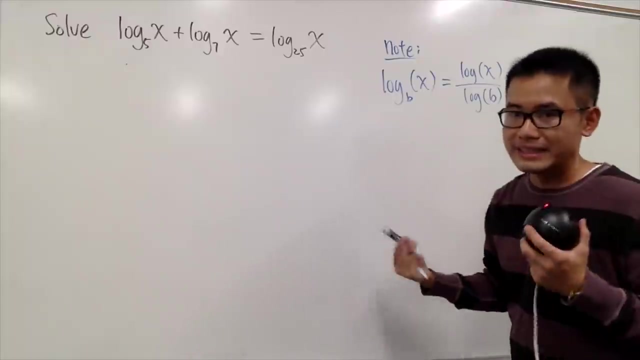 But why bother with that? And just to demonstrate how to solve this, I will use this form right here. You can have done the same with this, but it doesn't really matter, So let's put it down right here, alright? So our first thing is we have to write this in terms of log of base 10, right? 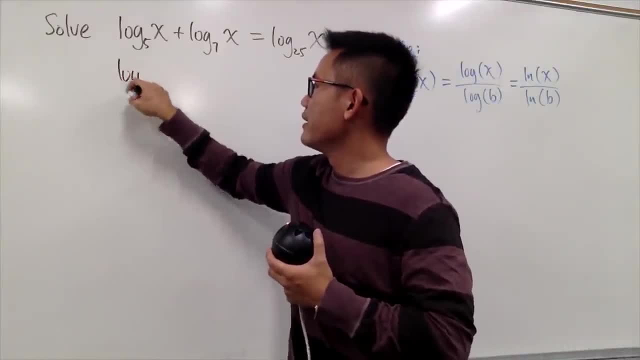 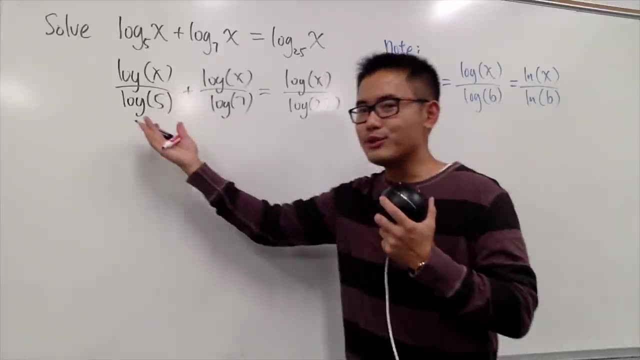 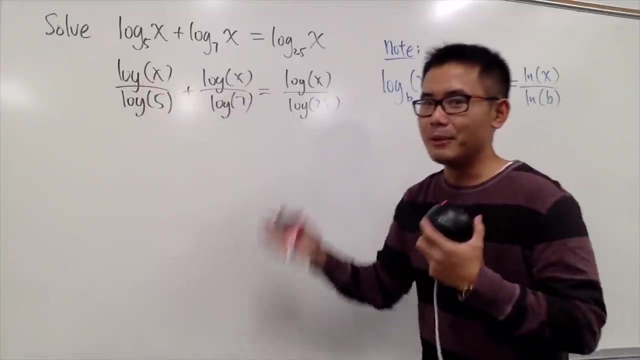 For the first term we will have log and the input is x over log of 5 on the bottom, like this. And you see, as long as you are doing this consistently, it's okay. Do not put down log log right here and then put down ln, ln. then you defeat the whole purpose of changing the face, alright. 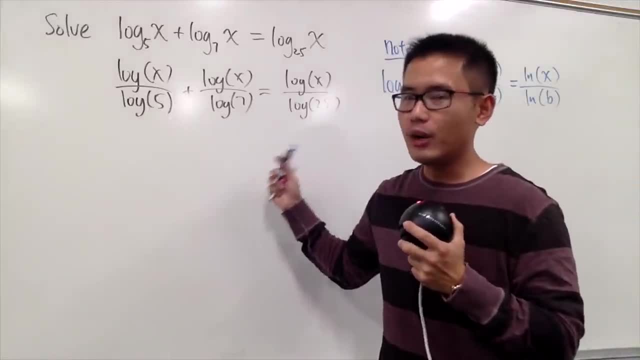 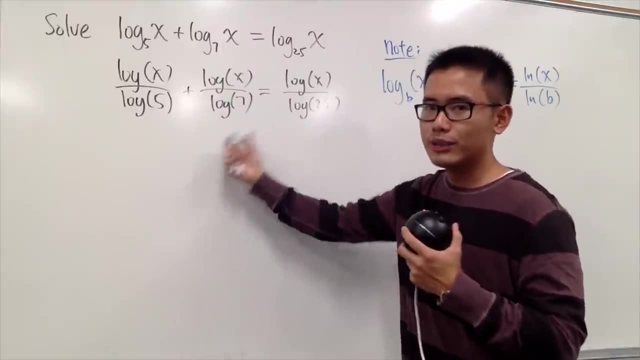 And now, as you can see, all of these three terms, they all have a log of x, right. So what we'll do is we'll move this from the right to the left and then we'll factor out the log of x. 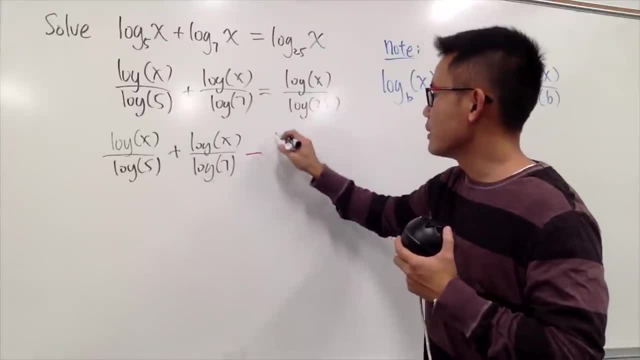 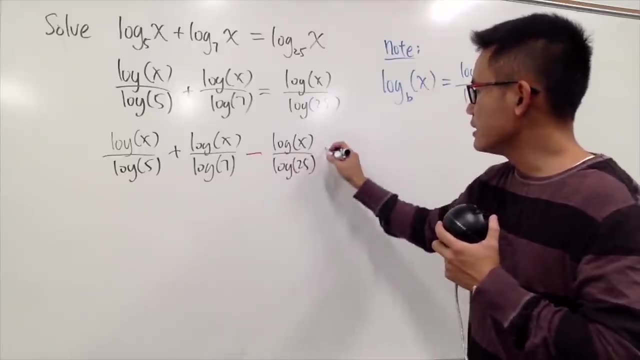 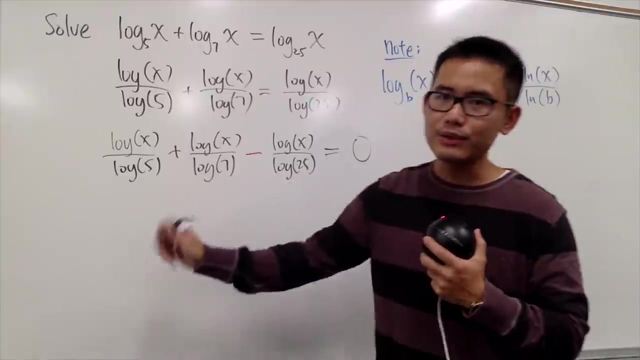 But let me move this for you guys. first It becomes negative, right. So we have minus log of x Over log of 25, and all this it's equal to 0. And now, as I said earlier, because they all have the log of x, we can factor that out. 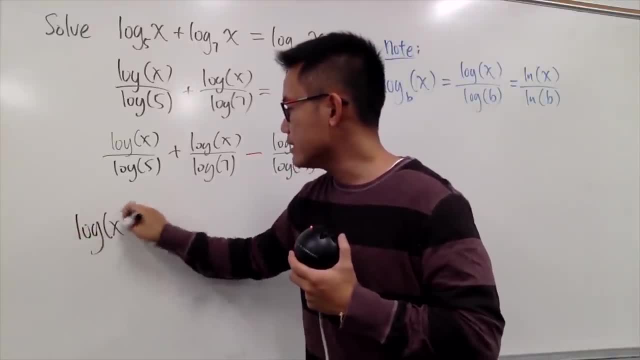 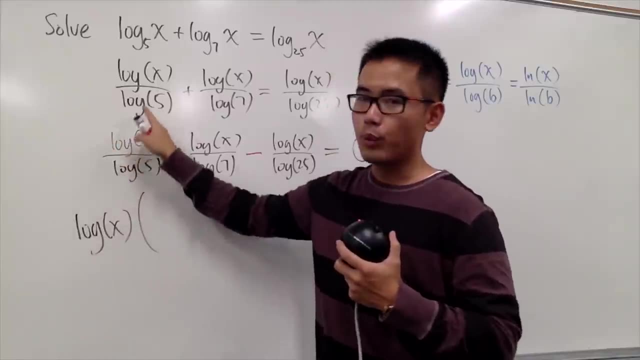 So let's do that, Let's put down the log of x all the way in the front and then open a bigger parenthesis. So here we factor out the log of x, so we have the 1 on the top. 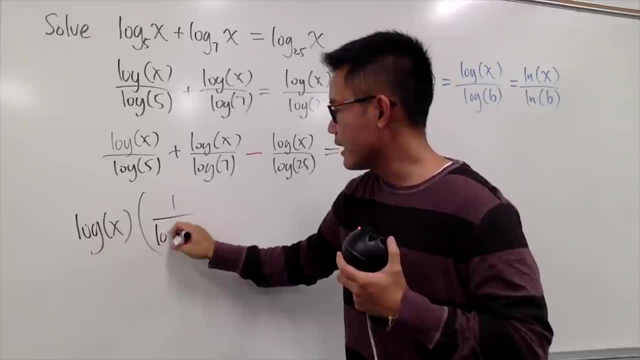 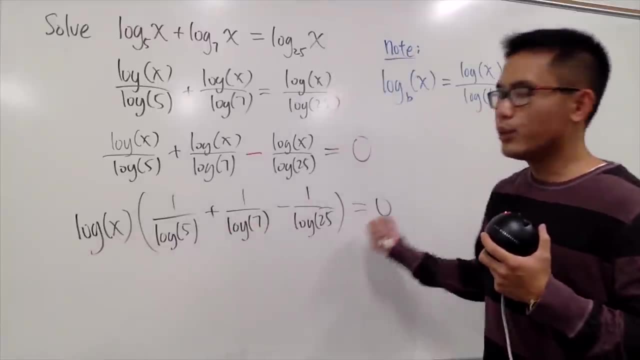 For the first term, we will have 1 over log of 5, like this: This is equal to 0.. Well, as you can see, we have log of x times this. it's equal to 0.. What is this? 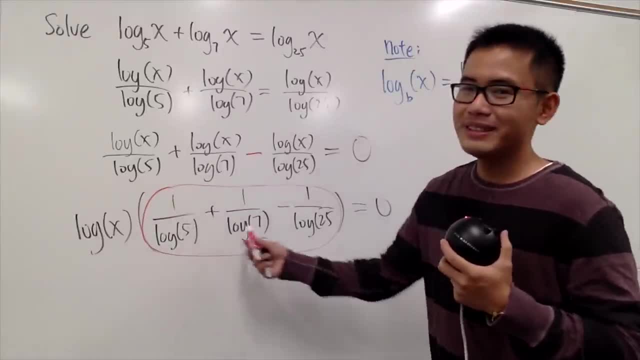 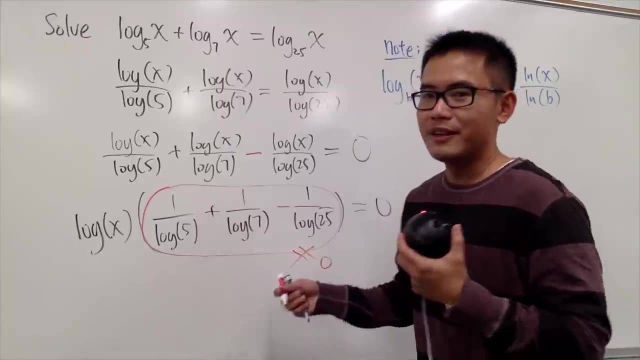 Well, you can try if you may, but no matter what you do, right here, this is not 0.. This is not 0, okay, Because well, just you can get a common denominator if you would like, and then, no matter what you do, just this is not equal to 0. 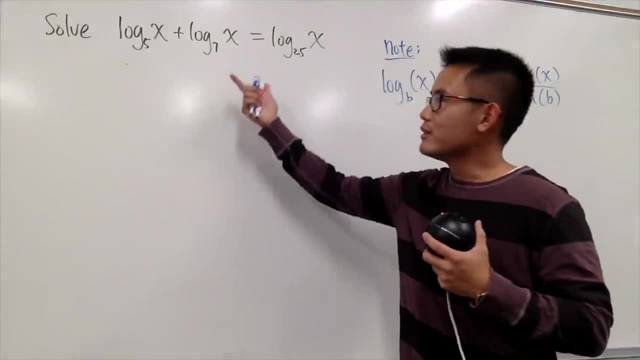 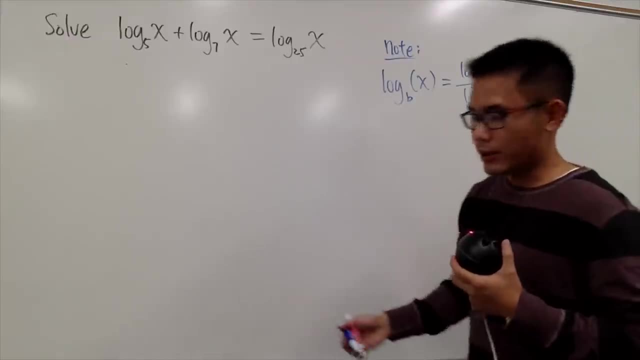 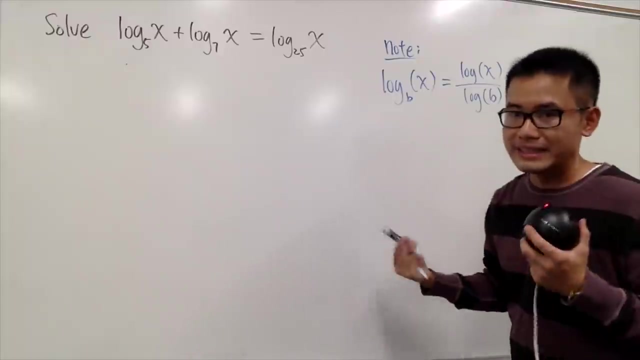 But why bother with that? And just to demonstrate how to solve this, I will use this form right here. You can have done the same with this, but it doesn't really matter, So let's put it down right here, alright? So our first thing is we have to write this in terms of log of base 10, right? 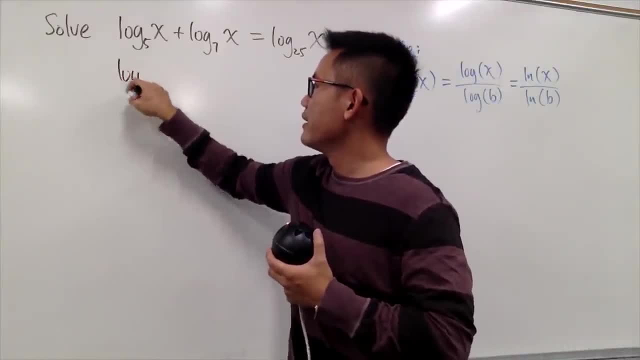 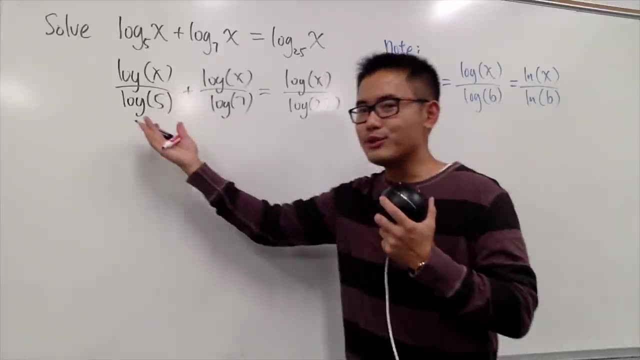 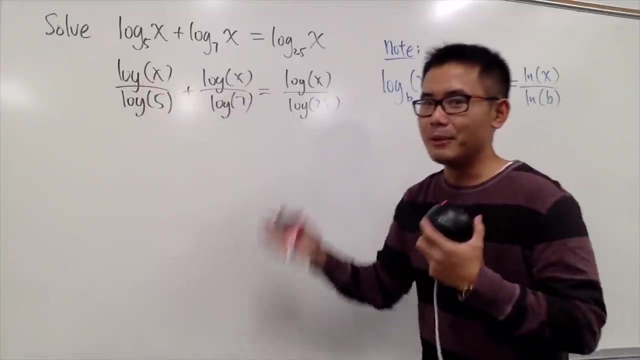 For the first term we will have log and the input is x over log of 5 on the bottom, like this. And you see, as long as you are doing this consistently, it's okay. Do not put down log log right here and then put down ln, ln. then you defeat the whole purpose of changing the face, alright. 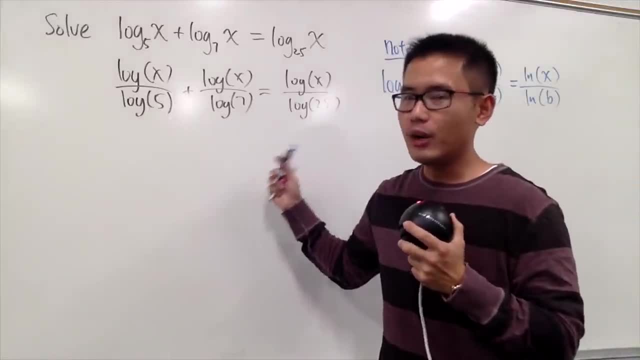 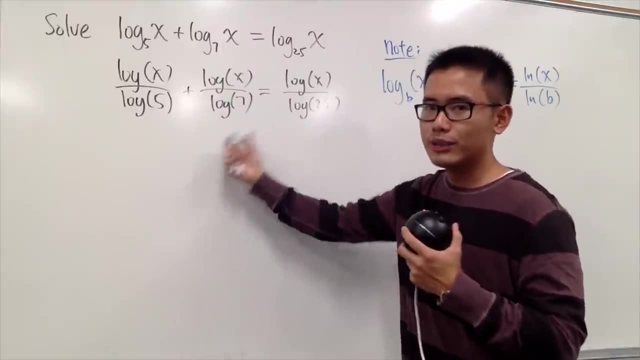 And now, as you can see, all of these three terms, they all have a log of x, right. So what we'll do is we'll move this from the right to the left and then we'll factor out the log of x. 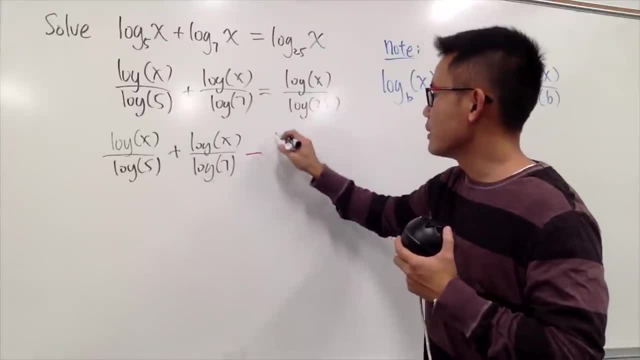 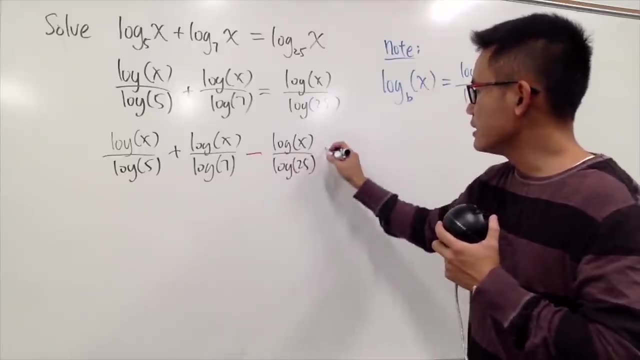 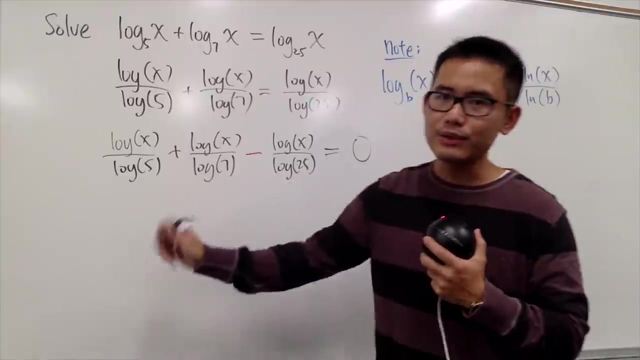 But let me move this for you guys. first It becomes negative, right. So we have minus log of x Over log of 25, and all this it's equal to 0. And now, as I said earlier, because they all have the log of x, we can factor that out. 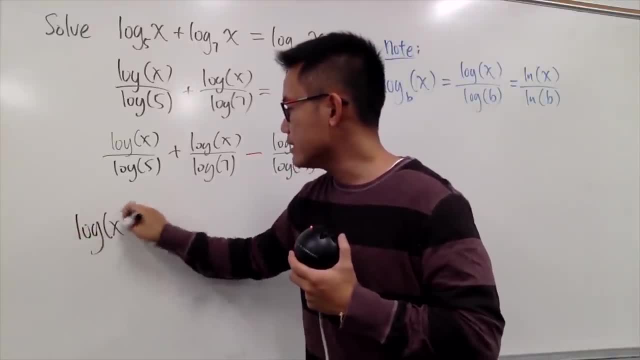 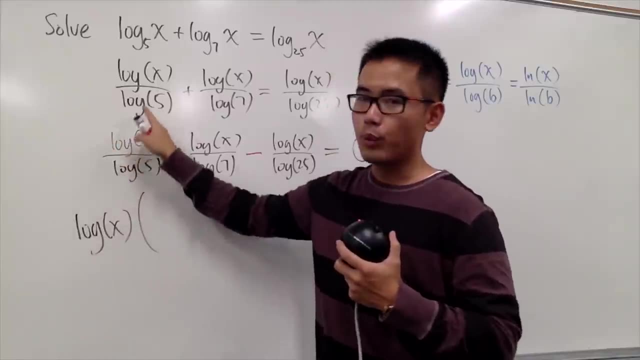 So let's do that, Let's put down the log of x all the way in the front and then open a bigger parenthesis. So here we factor out the log of x, so we have the 1 on the top. 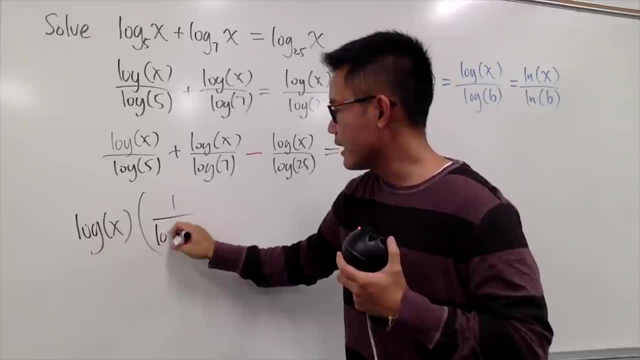 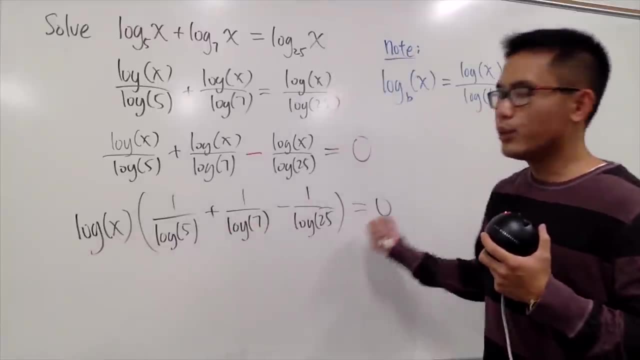 For the first term, we will have 1 over log of 5, like this: This is equal to 0.. Well, as you can see, we have log of x times this. it's equal to 0.. What is this? 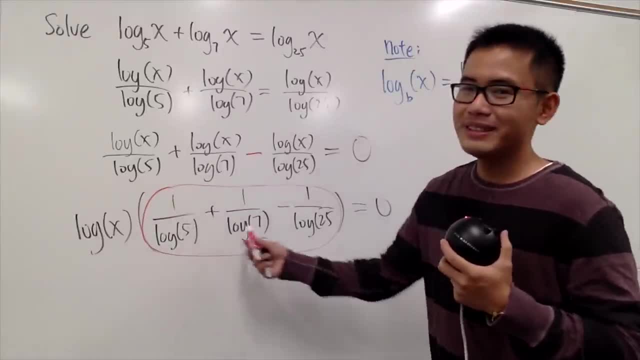 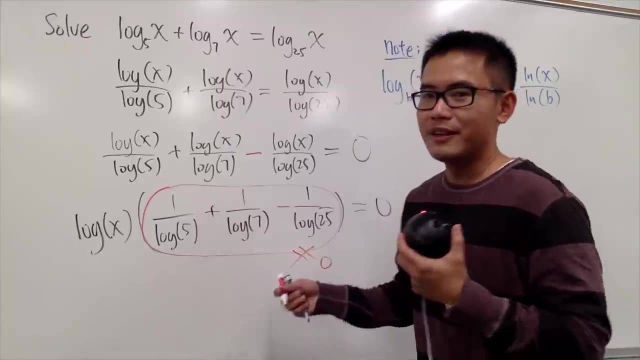 Well, you can try if you may, but no matter what you do, right here, this is not 0.. This is not 0, okay, Because well, just you can get a common denominator if you would like, and then, no matter what you do, just this is not equal to 0. 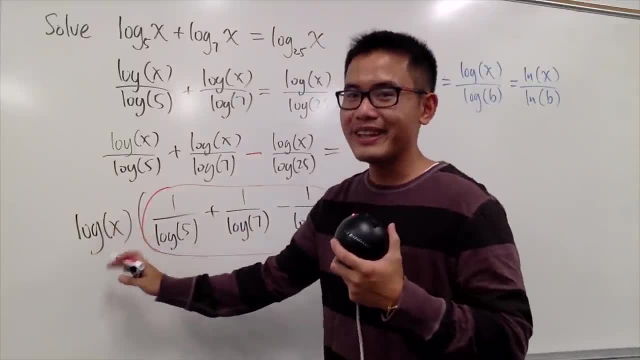 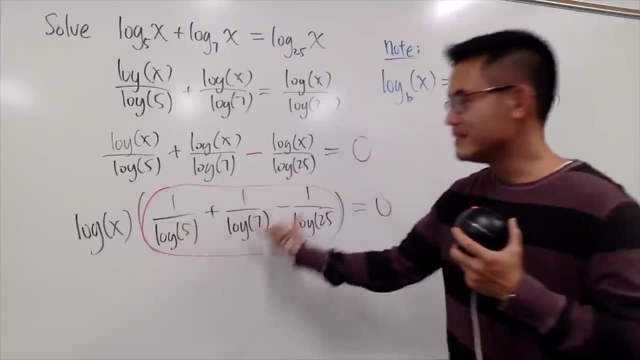 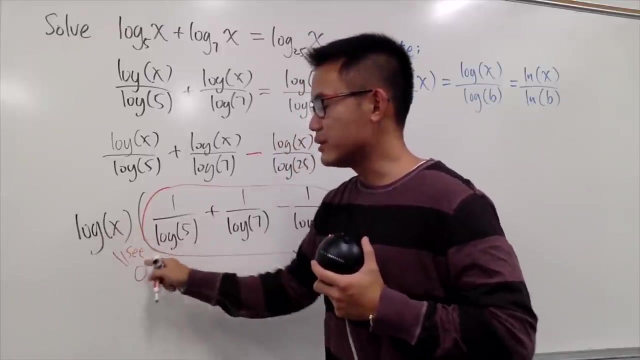 So the only situation to make this equation true- in fact here is the only place that has the x right- We have log of x times this non-zero number. that means we must have this equal to 0. So we have to set log of x equal to 0, so let's do that right here. 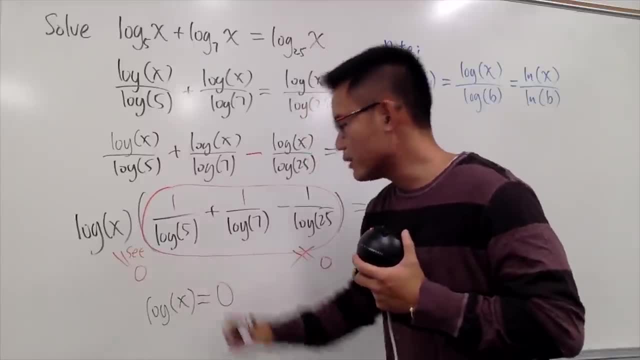 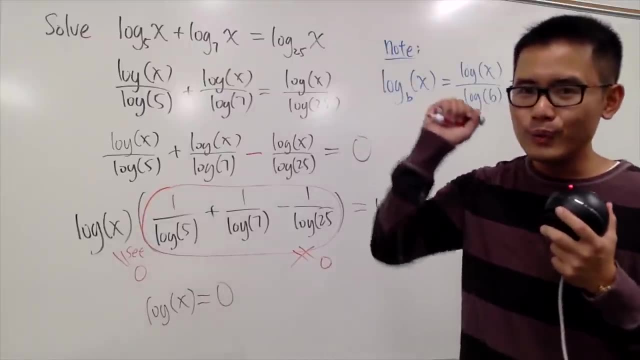 We must have log of x equal to 0, and now you have to ask yourself: log of what would be 0?? x has to be what. x has to be 1, okay, Another way to do it is that you know this is log. technically, we would say: 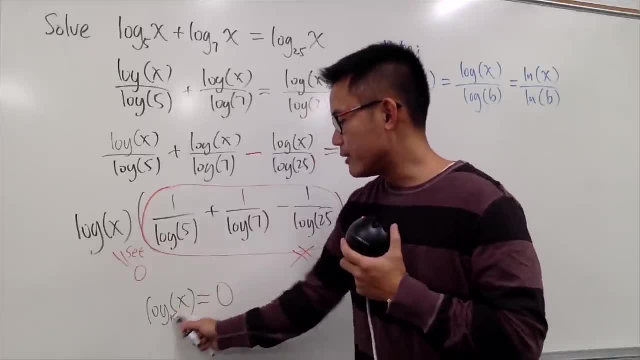 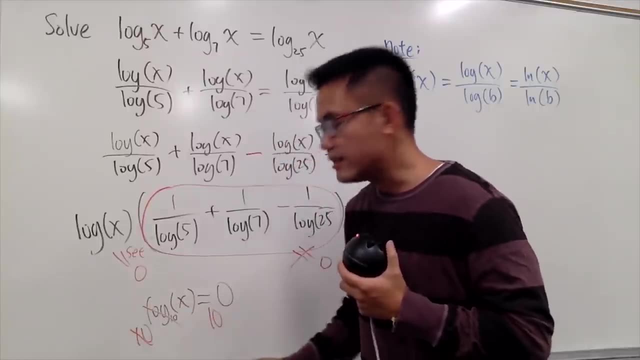 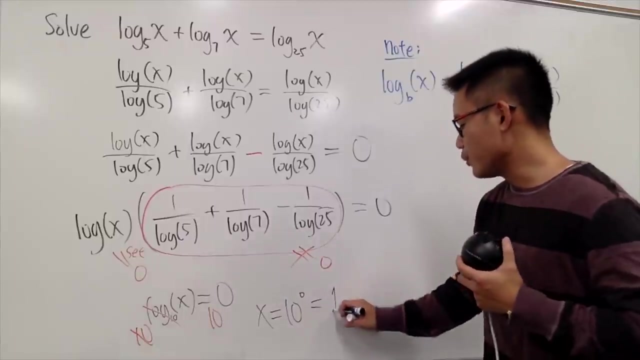 it's a base 10, and what we'll do is we'll pretend both sides are the exponents and we do 10 to this power and we do 10 to that power, so that this and that will cancel and we will have x to be 10 to the 0 power, namely, of course, it's just going to be 1, right. 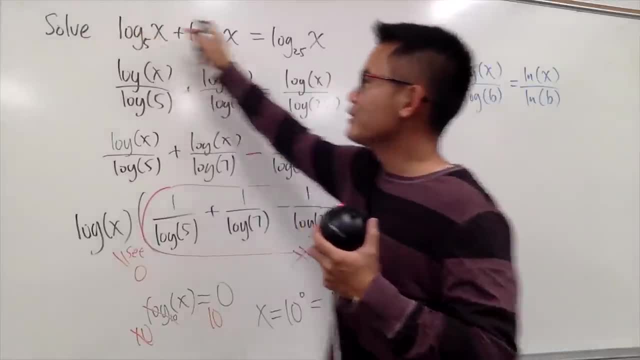 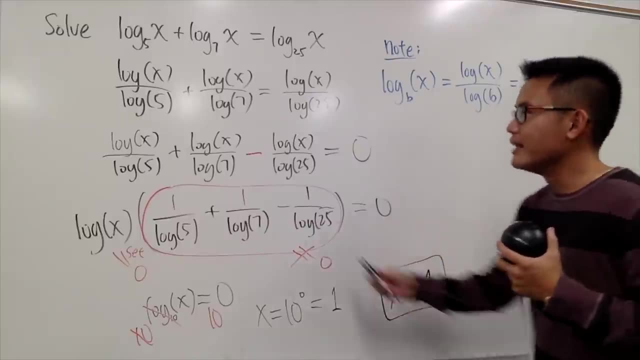 So, in fact, the answer to this right here, it's pretty trivial, in the sense that x is equal to 1, and when you plug in 1, all the x, in fact log base 5 of 1- is 0,. 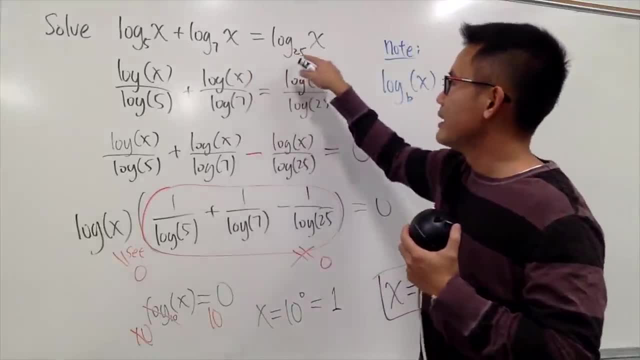 log base 7 of 1 is 0,. log base 25 of 1 is 0,. 0 plus 0 is of course 0.. 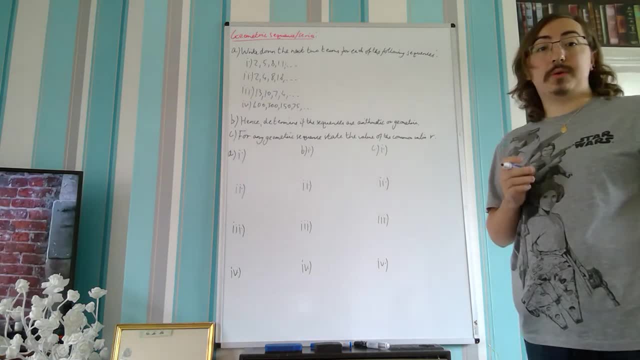 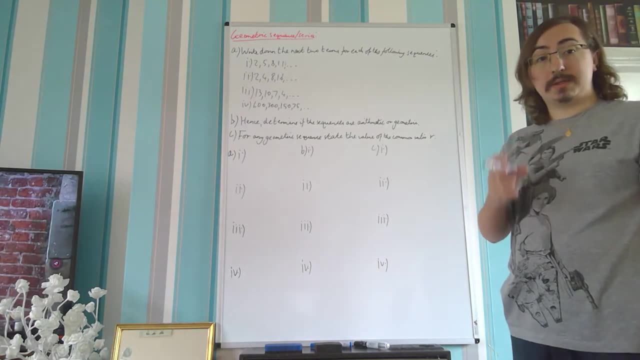 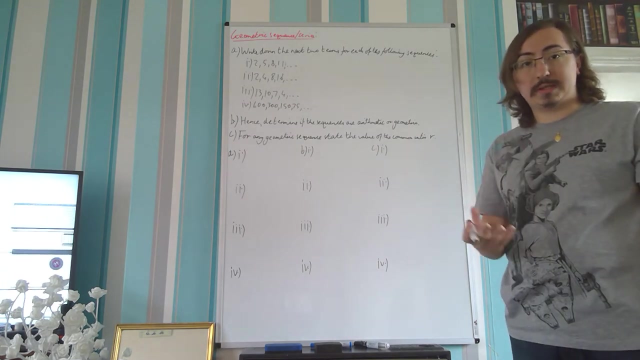 So in this video we're going to have a look at some arithmetic and geometric sequences Now, we've previously looked at arithmetic sequences in one of our other playlists, and an arithmetic sequence is where you're either adding on or subtracting by a fixed amount. 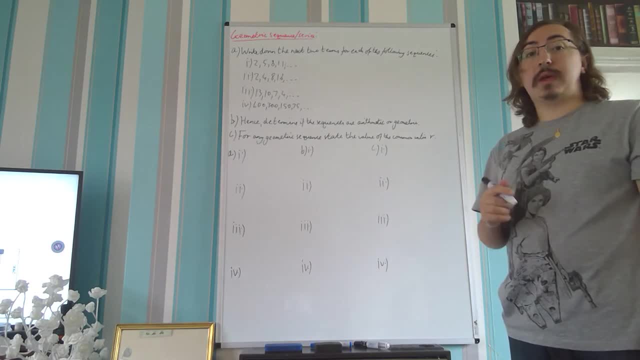 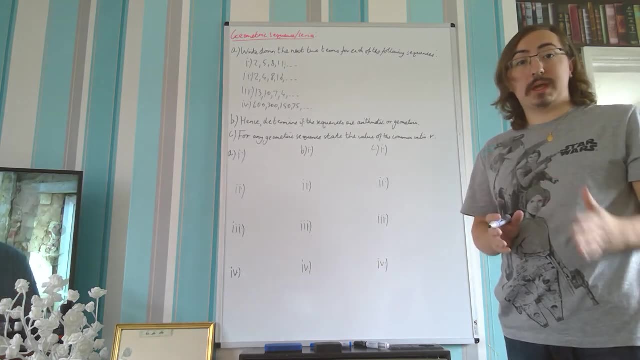 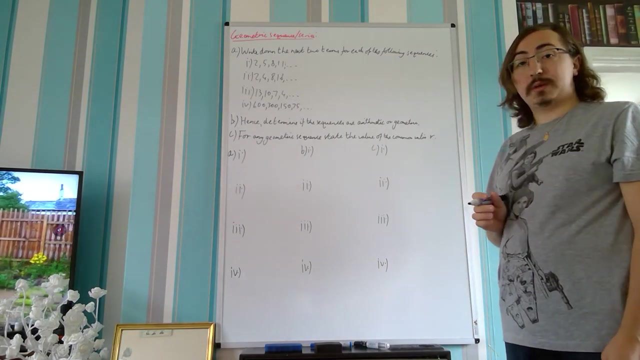 each time. Well, a geometric sequence is if you are multiplying from each term to the next, or dividing. but really we're going to treat it always as a multiplication, because you can rewrite a division as a multiplication. So for our first sequence, then part A says: 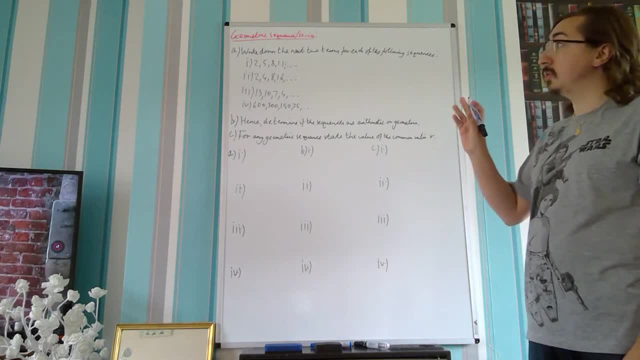 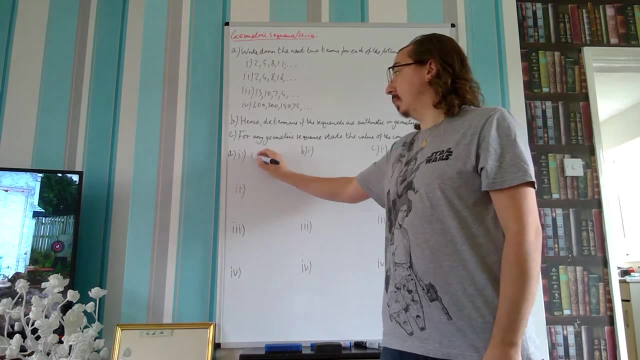 write down the next two terms for each of the following sequences. So we have 2,, 5,, 8,, 11.. What's happening each time? Well, we're adding on 3.. So our next two terms would be 14 and then 17.. Moving to sequence 2, then We have 2,, 4,, 5,, 6,, 7,, 8,, 9,, 10,, 11,, 12,, 12,, 13,, 14,, 14,, 15,, 16,, 17,, 18,, 19,, 20,, 21,, 21,, 21,. 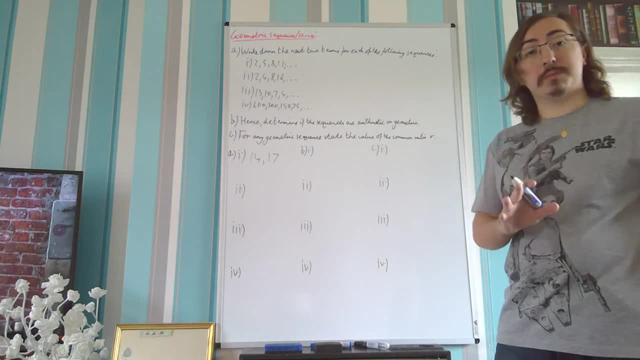 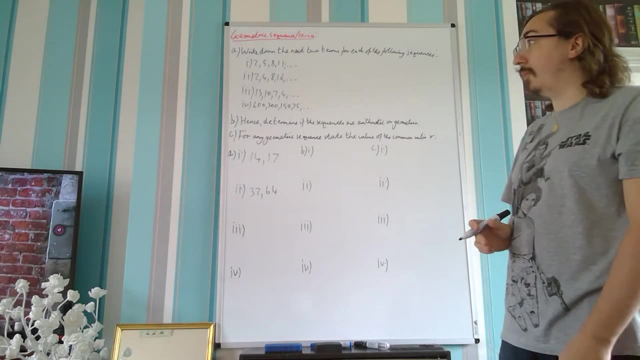 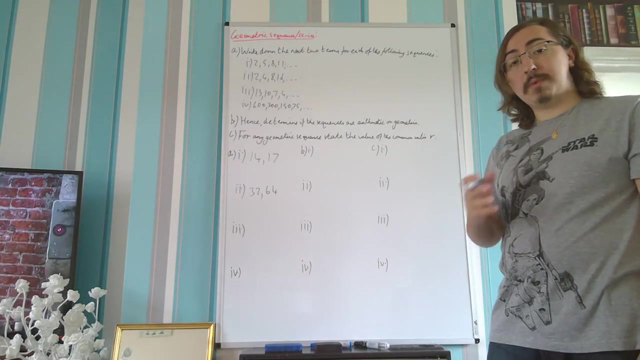 22,, 23,, 24,, 28,, 16.. What's happening each time? Well, we're multiplying by 2.. 16 times 2 is 32, and 32 times 2 is 64.. For the third sequence, we have 13,, 10,, 7,, 4.. What's happening this time? Well, we're.